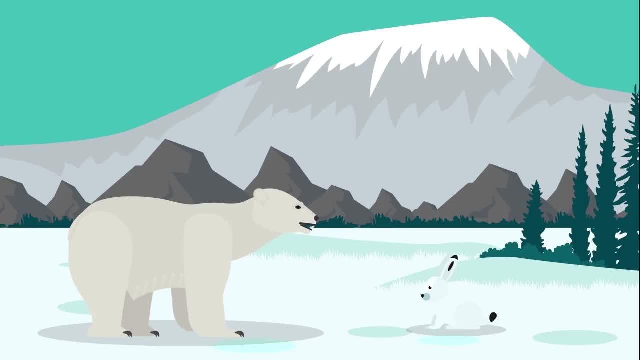 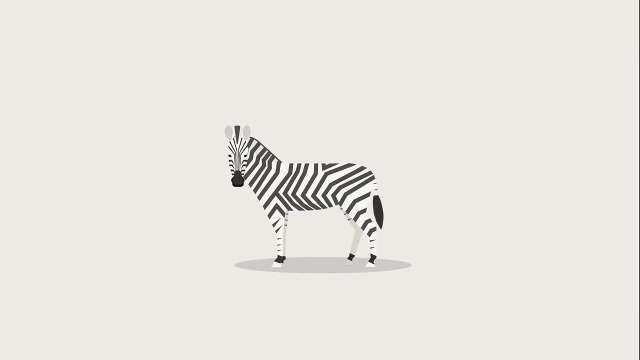 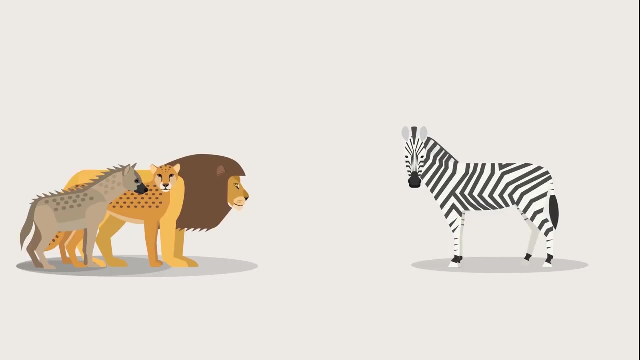 why most prey use unique colorization or complex patterns on their coat to blend in with their environment and keep concealed. For the zebra, an animal that shares a habitat with cheetahs, hyenas and especially the lion, this strategy would make sense. However, the high contrast 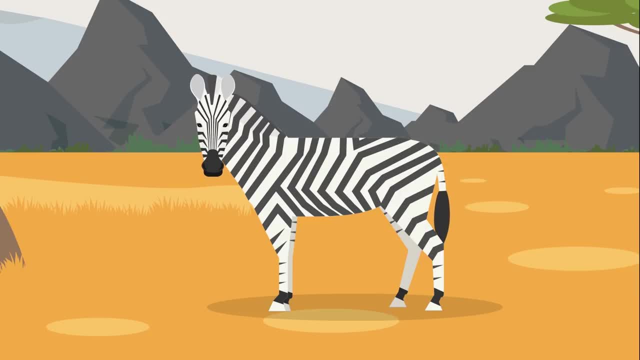 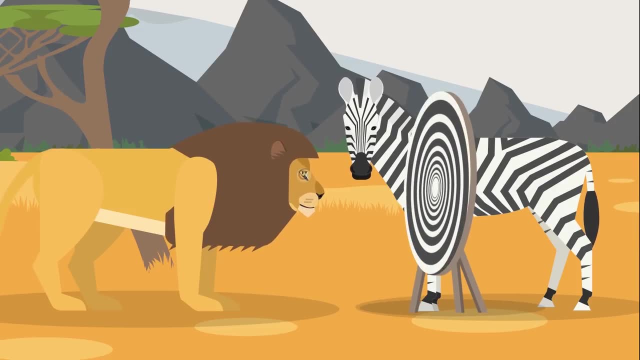 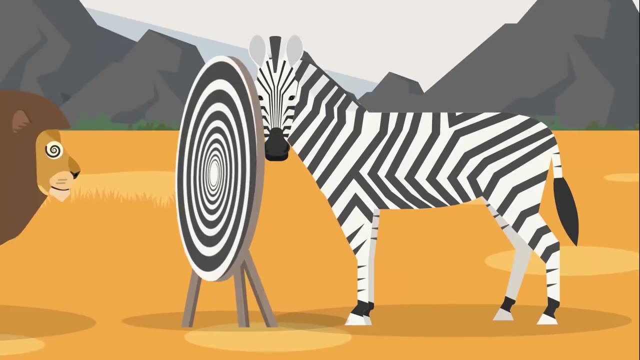 of the zebra coat seems to make running away a lot harder. them stand out more than blend in, especially against the plain savannah background. Another popular theory is that the stripes dazzle predators by making it more difficult for them to judge the zebra's size and speed. however, there's no evidence to support this. 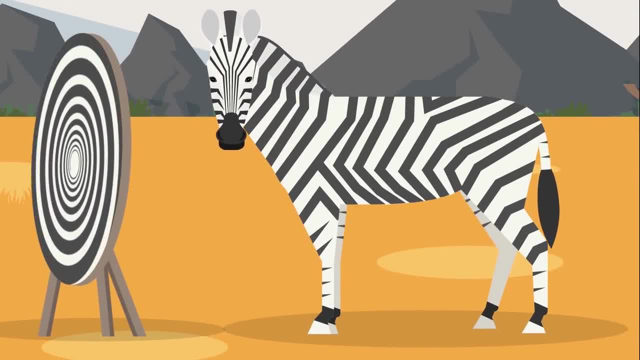 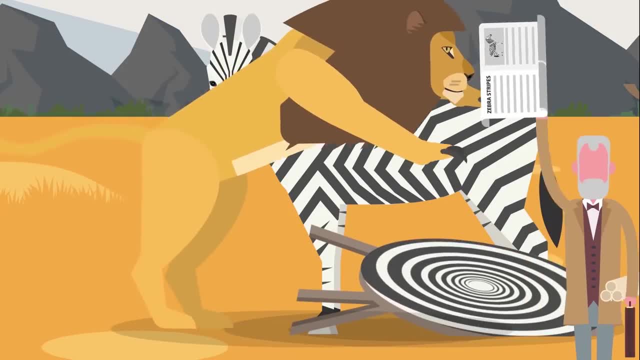 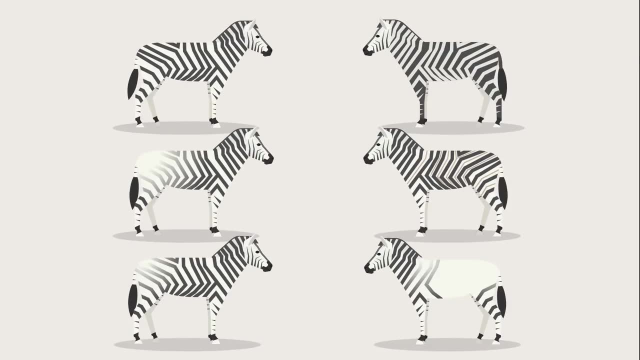 theory. Actually, quite the opposite seems to be the case. A study from 2015 done by researchers from the University of California found that the zebra's main predator is particularly good at catching zebras. By examining the different stripe styles of zebras at 16 different sites from South to. 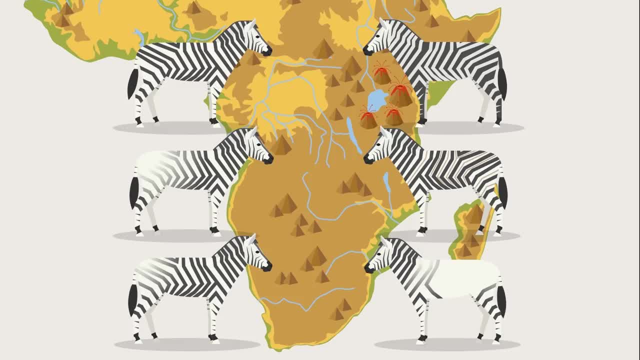 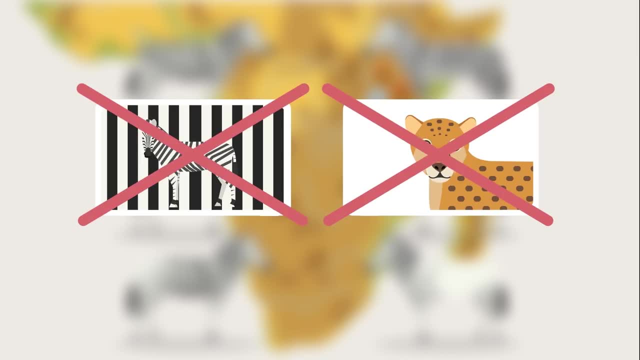 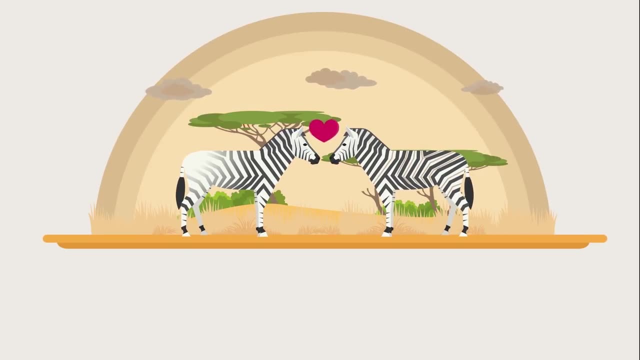 Central Africa. the researchers also couldn't find any link between striping and lion populations, which seems to eliminate both previous theories definitively. The theory that the stripes help zebras recognize each other is certainly plausible, but it's unlikely that zebras will recognize each other. 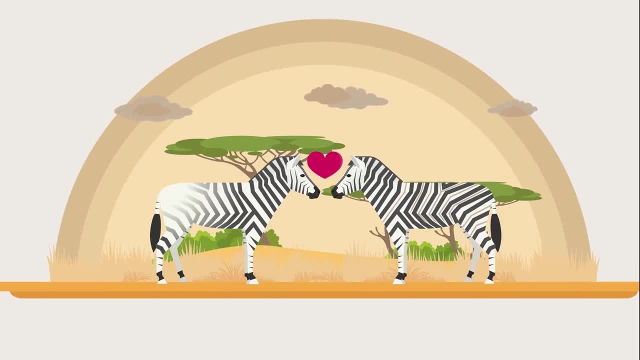 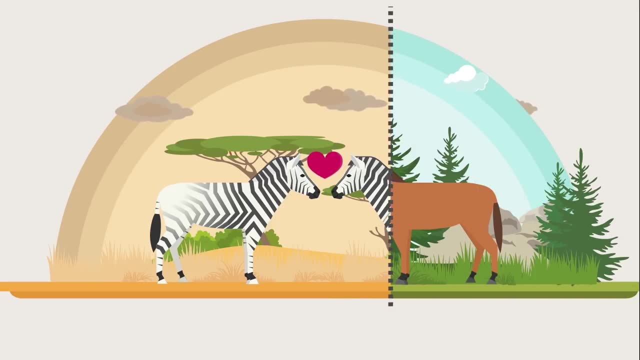 Such complex patterns evolve. just for that purpose alone, It should take less than a full-body barcode for zebras to tell each other apart. Wild horses live in social groups as well, and they have no issues doing so, despite being single-colored. Luckily, the study found more. 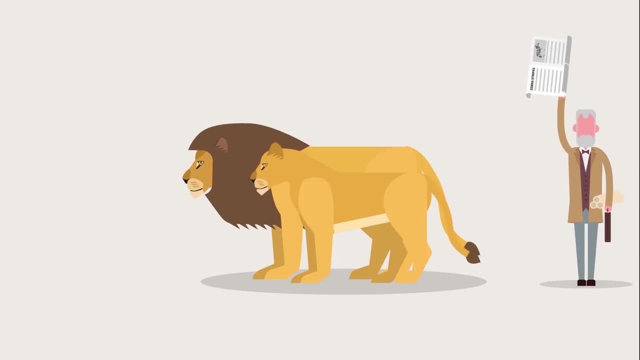 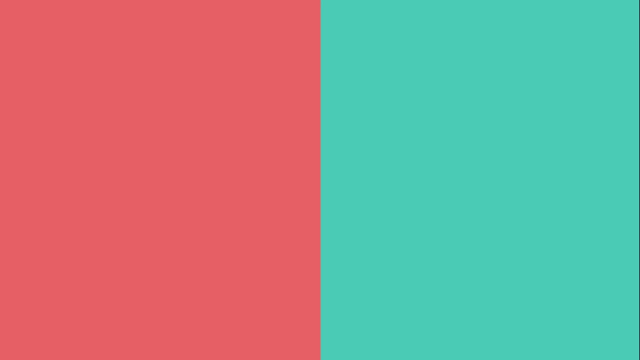 Not only did they compare the different stripe styles to lion populations, but to 29 different environmental factors. The only two factors that showed a significant correlation were temperature. temperature and temperature: These findings support two entirely different theories. The stripes could play an important role in keeping the zebra cool in the African heat. 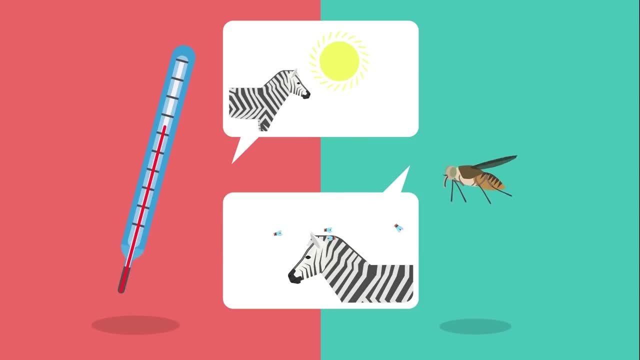 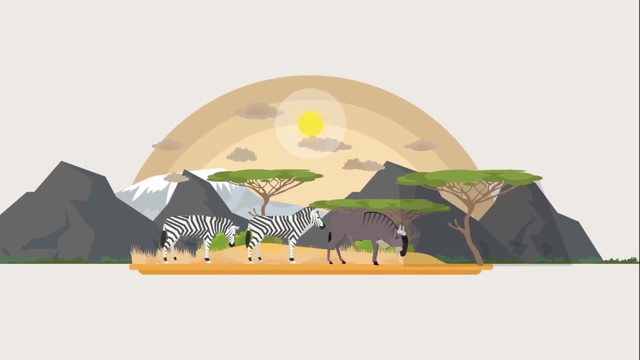 or perhaps they are there as a protection against disease-causing flies that are especially common in the hottest climates. Zebras digest food much less effectively than other grazers in Africa. As such, zebras need to spend longer periods of time in the wild. 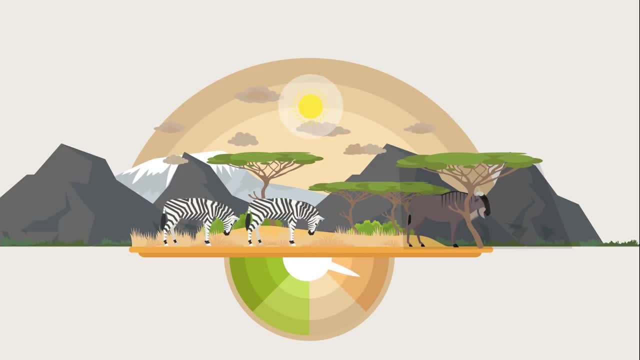 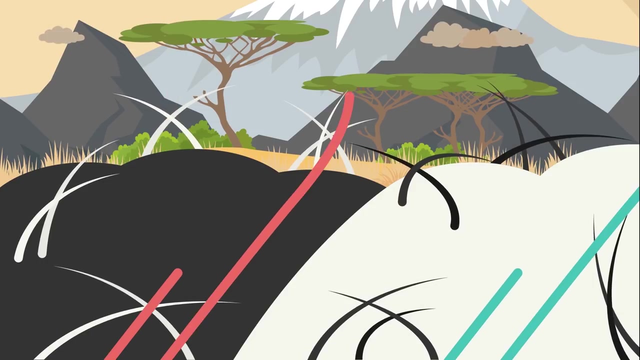 They eat more food in the heat of the midday sun. This could make an additional cooling mechanism necessary, which may explain why the stripes of zebras in hotter regions are more pronounced. In theory, the currents of air that flow over the zebra's body are faster over the black. 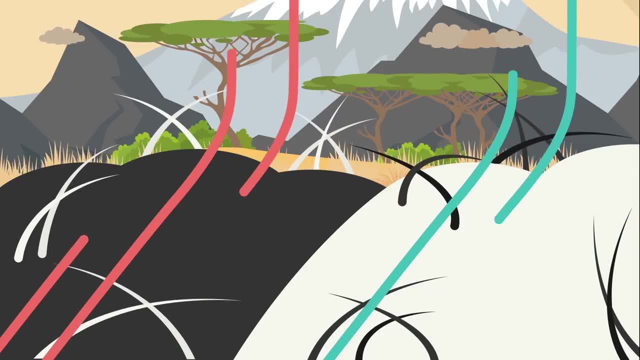 parts, since black absorbs more heat and slower over the white. At the juncture of these air flows, the air may create little swirls to cool down the zebra. Still, the researchers have not yet experimentally tested this theory, but there is evidence. 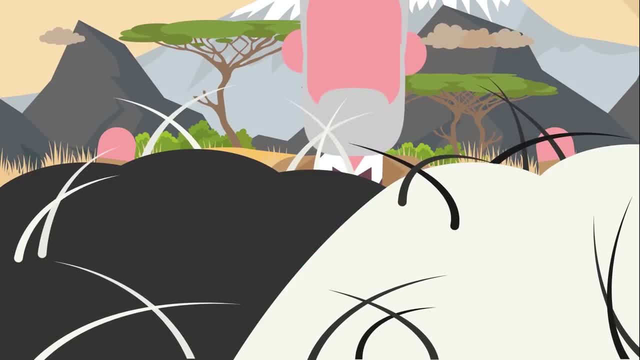 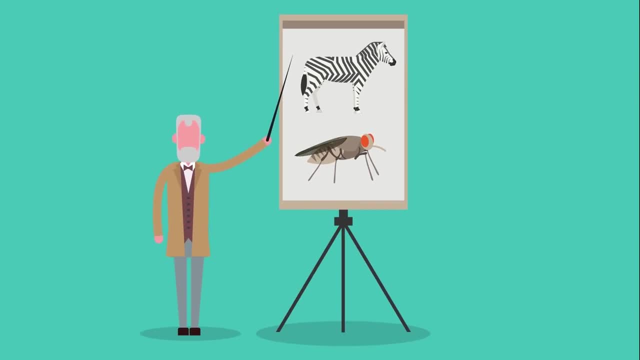 as heavily striped zebras have lower skin temperatures than other non-striped mammals in the same area, But the findings could also be interpreted differently. In 2012,, the BBC reported that a study from researchers from Hungary and Sweden drew a link between the zebra stripes and the occurrence of blood-sucking flies carrying deadly diseases. 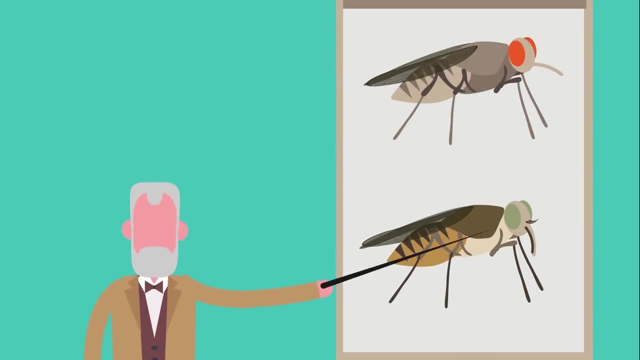 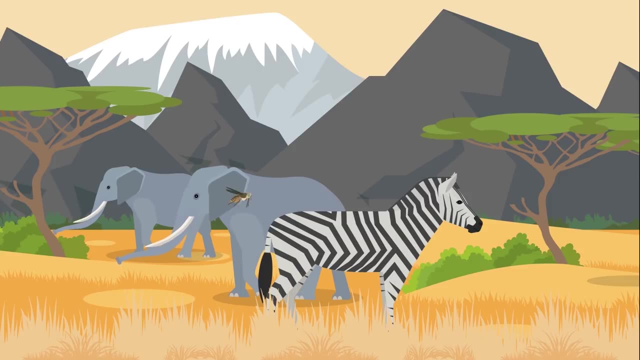 The researchers also found that the blood-sucking flies are more likely to cause diseases than the zebra. Both tsetse flies and horseflies are vectors for significant and often fatal diseases in horses. The zebra's short hair and thin skin would make it especially susceptible to bites necessitating 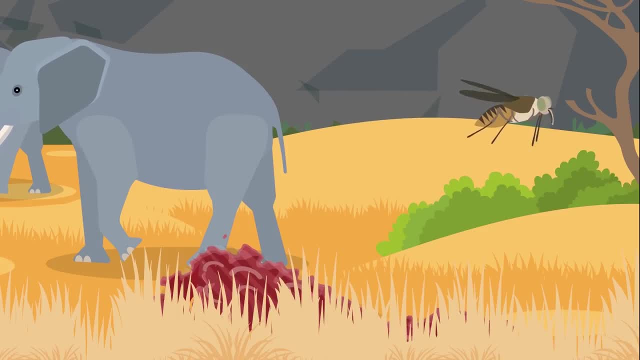 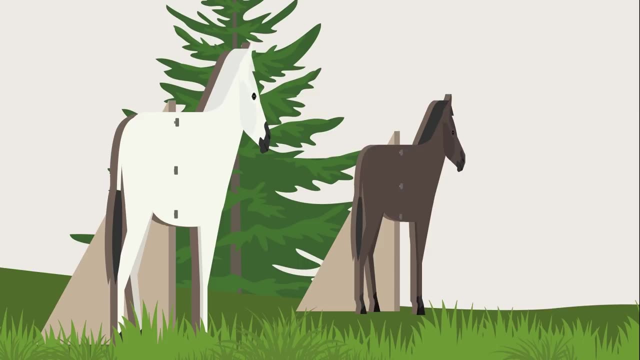 the need for extra protection against these insects, Especially in the hotter regions, where they tend to be more common. In a practical test, the researchers could successfully show that different-colored coats repel flies more or less successfully. That is because flies are especially susceptible to blood-sucking flies. 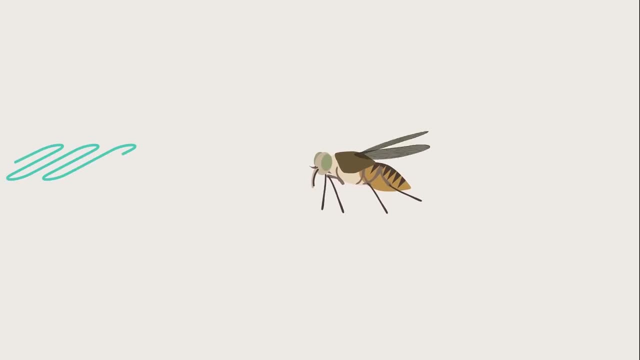 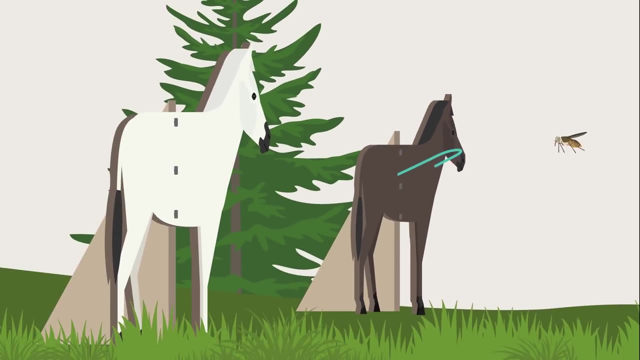 These flies are especially attracted by polarized light that moves along a horizontal plane much like a slithering snake. These waves are created when light bounces off dark surfaces, which makes dark-colored horses, for example, very attractive to flies. The unpolarized light that bounces off white coat travels along any and every plane making. 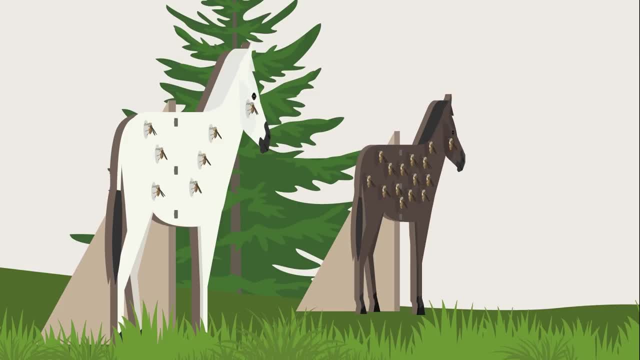 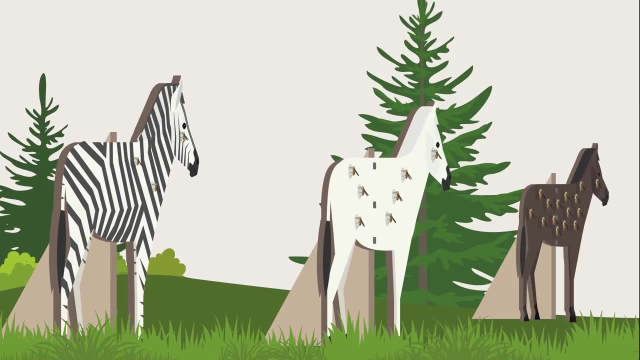 white-coated horses much less attractive to insects. Astonishingly, zebra-like stripes tend to be more likely to cause diseases than other animals. These stripes, despite being partially dark, were the least appealing to flies during the tests, and even though scientists have not quite figured out why that is, it could explain.